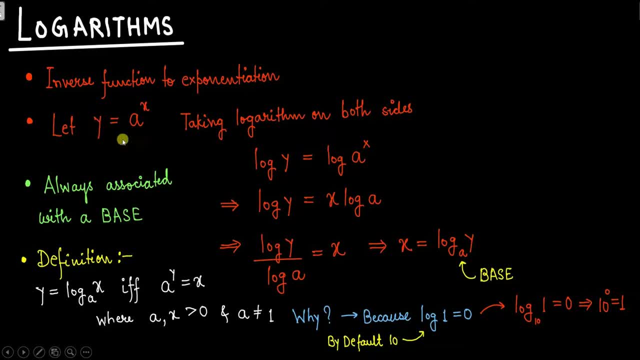 Can you see this? On the left hand side it's y, So y is written here, a to the power of x is written So a to the power of x. So simply I have taken log on both the sides. So here I have taken log. 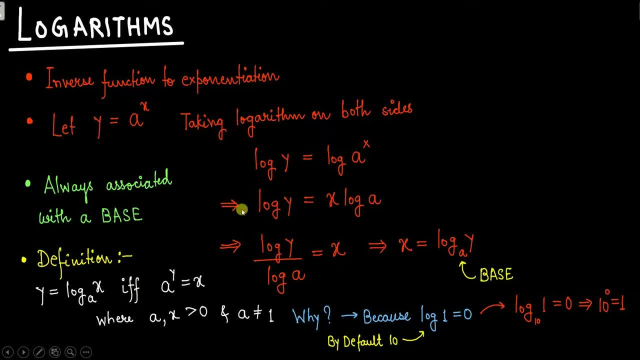 now. this implies log y equals to now. this is the rule that whatever is there in the power, so that gets multiplied with that. Okay, so here if it is x, so this x will be getting multiplied on the left hand side. Fine, so this could be written as: log y equals to x, log x- Okay now. 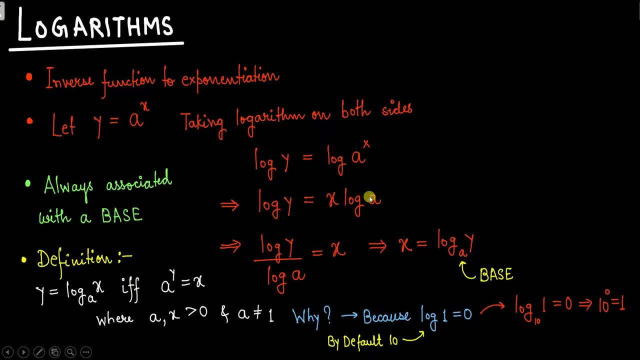 log y and here it's log a. So bring this log a down. So here you can write again: log y equals to log a. Okay, which is equal to x. So here you can write this as x equals to log y to the base a. 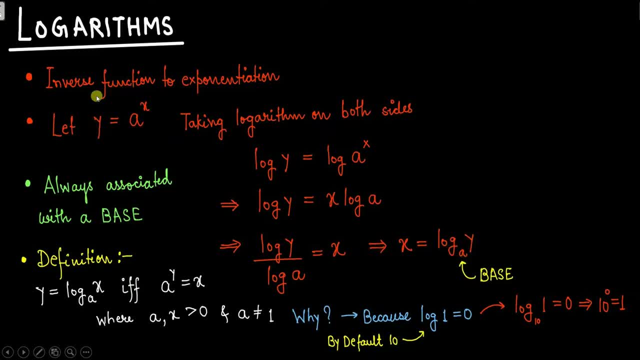 Now see, initially it was y equals to a to the power of x. So this has been converted into: x equals to log y to the base a. Okay now, what is the rule to remember? So whenever you find anything written like this, simply you just take this as the base and on that. 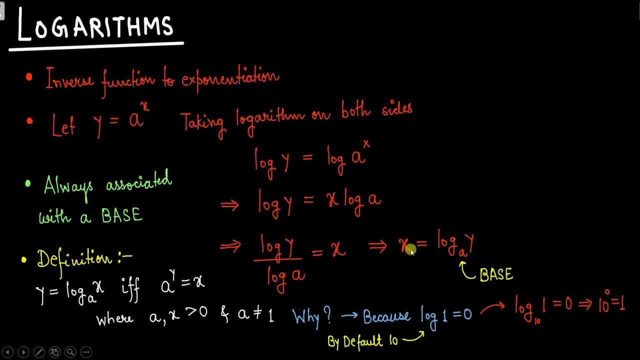 power. x is being headed on the power, So this could be written as: y equals to a to the power of x. Okay, so y equals to a to the power of x could be written as: x equals to log, y to the base a. Okay, so here this a is called as the base. Fine, so log is always associated with a base. 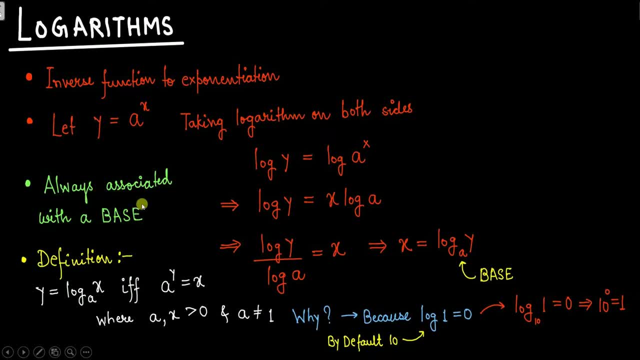 Log is always associated with a base. You cannot define any logarithm without a base. A base has to must thing to happen. Okay, so a logarithm always associated with a base. So what is the basic definition for this? So y equals to log, x to the base a. So this is only possible if a to the power. 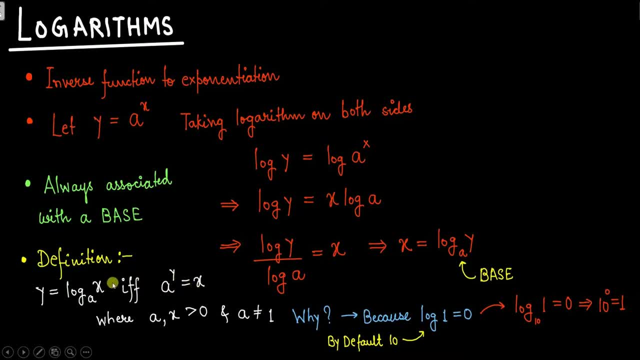 of y equals to x. Now see, this is a mathematical language. Don't think that I have done a spelling mistake out here. So this is not a spelling mistake, It is a mathematical language of writing if and only if. Okay, so I double f means if and only if. So if and only if. a to the power. 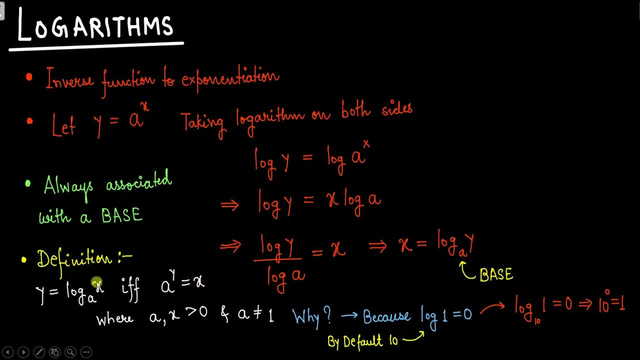 of y equals to x, then only you can write this as y equals to log x to the base a. Fine, provided your a and x has to be 0.. Your a and x has to be 0. And a is not equal to 1.. So this base a should. 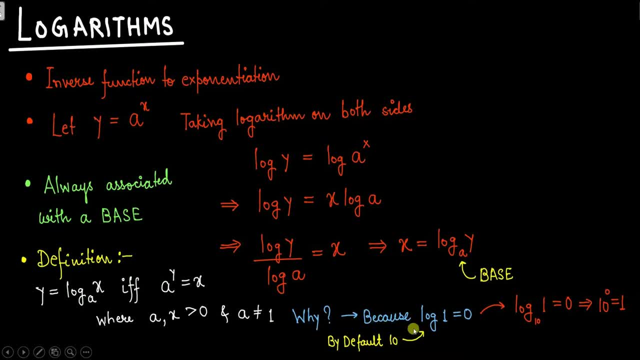 not be equal to 1.. Why? Because we know that log 1 is 0.. Okay, log 1 is 0. Now here you will ask me, sir, here you have not given any base. Then, dear student, remember that if nothing is mentioned, then by default the base is considered as to be 10.. 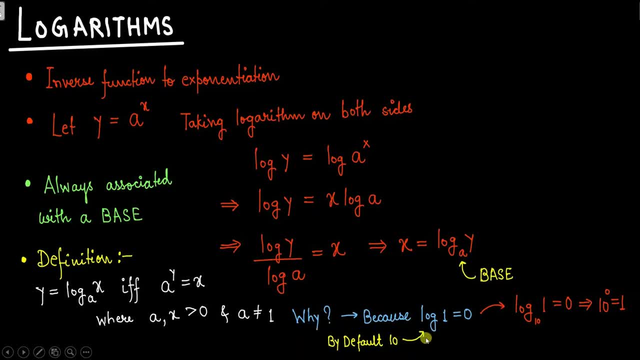 Then by default the base is considered as 10.. Okay, so here I am writing: log 1 is equal to 0. So if log 1 could also be written as log 1 to the base, 10 equals to 0 equals to 10 to the power of. 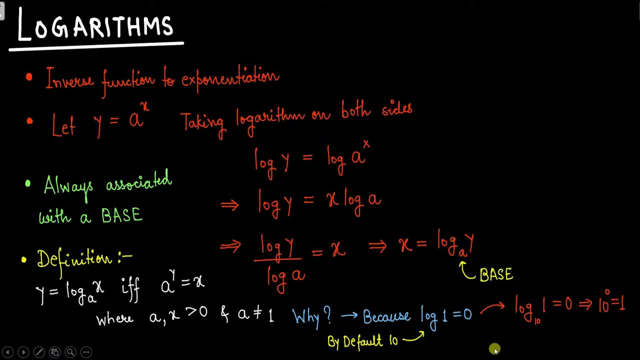 0 equals to 1.. Okay, so here you can write: log 1 equals to 0.. Now we know that log x by log a. So in the denominator if log 1 comes. so in the denominator if 0 comes. so that makes the thing. 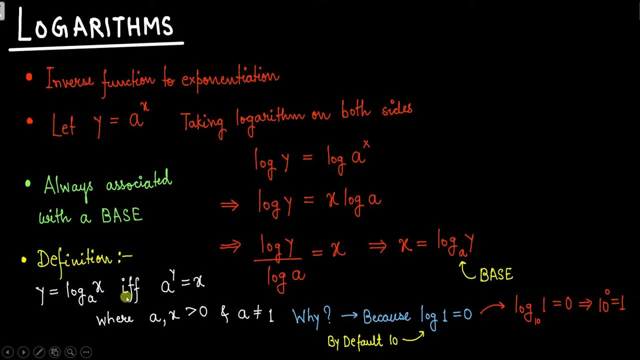 indeterminate. So that is why a, or the base a, should not be equal to 1.. Is this clear to you? Once again, let us have a quick recap. Logarithm is an inverse function to exponentiation. I can write: y equals. 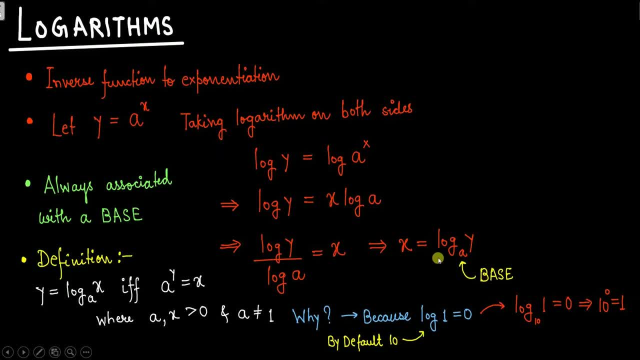 to a to the power of x, as x equals to log y to the base a And it is always associated with a base. So this is the basic definition. provided log 1 is equal to 0. So this 1 cannot be considered as the. 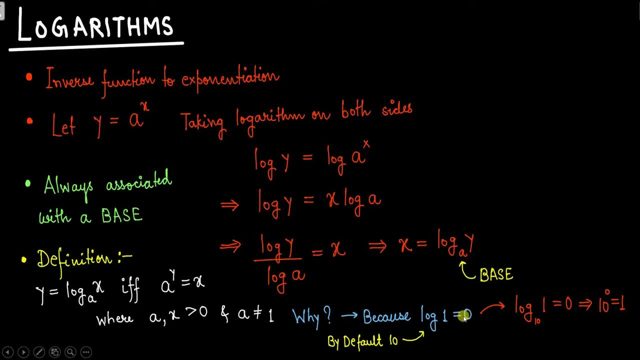 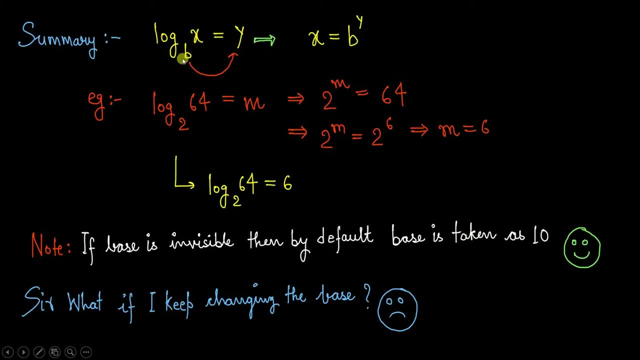 base 1 is never taken as a base: See the summary. So log x to the base. y equals to y. Okay, so what is the rule? So whatever is written here, so b, you can take this b here and in the power you bring y. So that will be taken as x. Okay, so this is the rule of 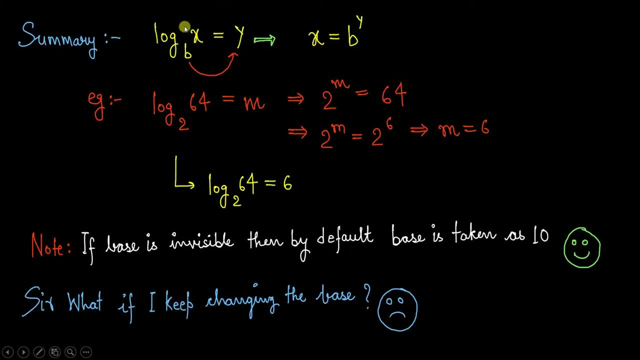 converting or removing the log. If you want to remove the log from this expression, you can write this manner: Okay, so x is equal to b to the power of y, x equals to b to the power of y, or x equals to b raised to the power of y. Let us see an example. So if something is written like this: 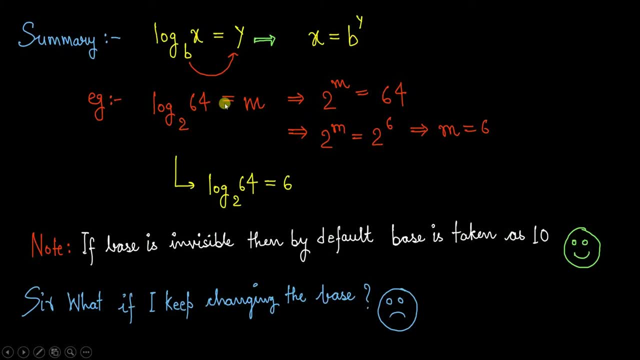 64 to the base 2 equals 2.. So we need to calculate this value. Fine, So let us assume that log 64 to the base 2 equals to m. So from here you can write: 2 to the power m equals to 64,, 2 to the power of m. 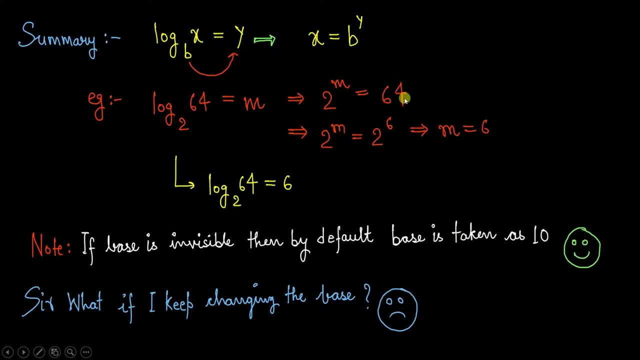 equals to 2 to the power of 6.. Why? Because 64 can be written in the power of 2.. Why I am doing this? Because in the previous class we had learned powers and rules. Remember So, in that we just 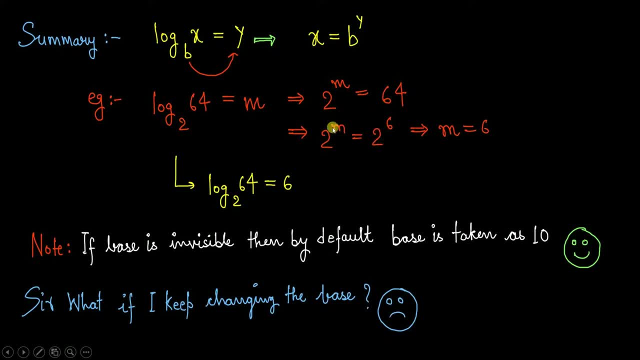 saw that whenever the base is same, the powers has to be the same. So we can write: 2 to the power of m equals to 2 to the power of 6.. Okay, whenever the base is same for this expression to be equal. 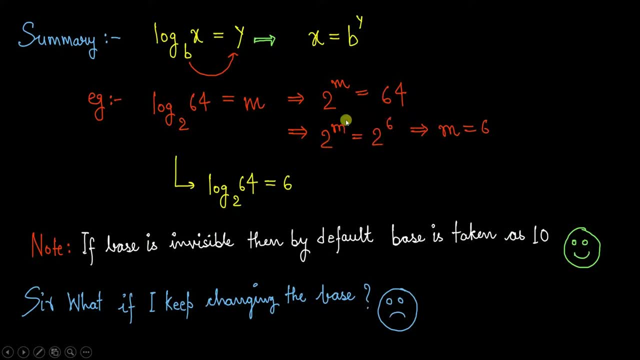 the powers has to be same, So 2 to the power of m. if this has to be equal to 2 to the power of 6, then definitely this m value has to be 6.. Okay, so from here we can write: here: m equals to 6.. 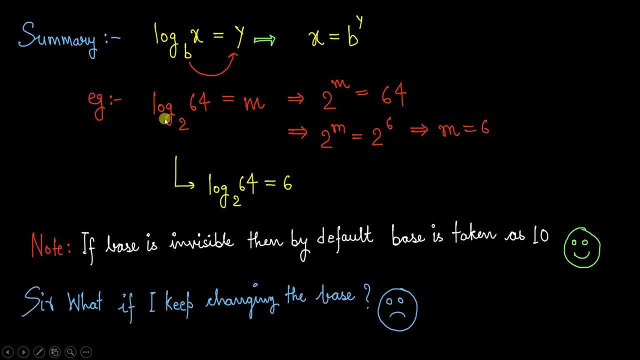 So finally we got an answer for this. That is, log 64 to the base. 2 could be written as 6.. Fine, There is a note. If the base is invisible, then by default the base is taken as 10.. Just now I had told you: if base is invisible, then by default the base is taken as 10.. 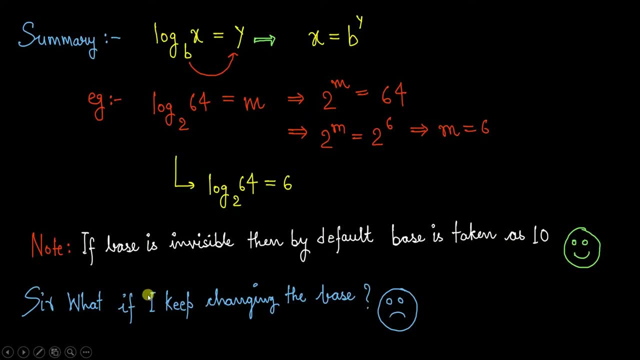 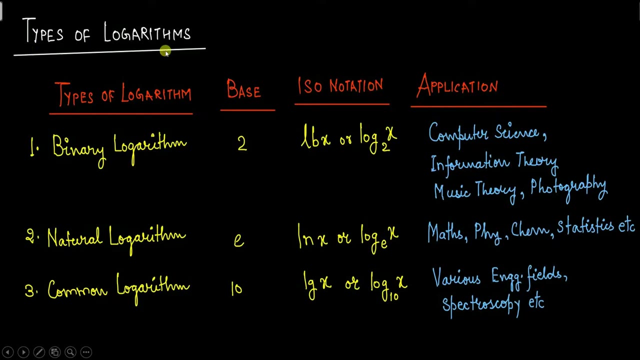 Now you will be having one question, Sir: what if, if I keep changing the base, can I have any other base other than 10?? Then your answer is here. So we have different types of logarithms. Let's have a look on this. We have different types of logarithms, So I have 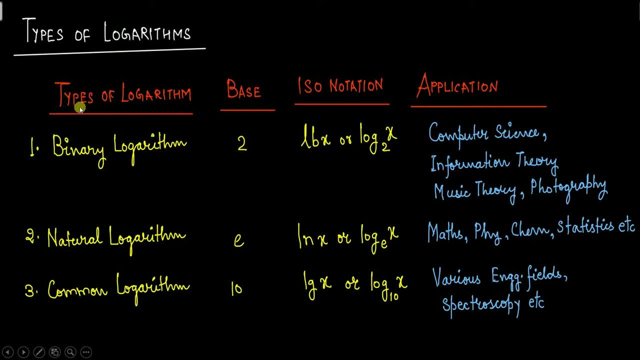 written this nicely. So this is the types of logarithm, the base. What is the ISO notation? Do you know what is ISO? Just Google it out. It is International Organization for Standardization. Okay, So ISO has given some standard notations that we need. 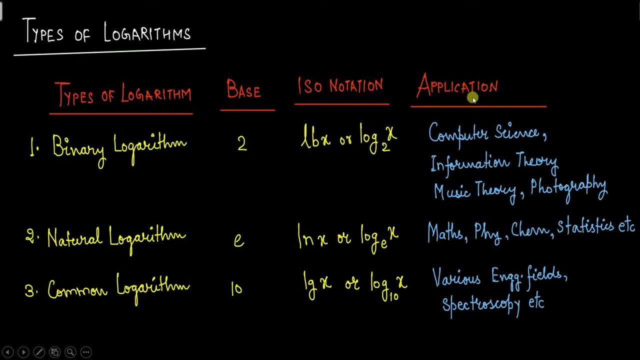 to follow And what are the applications? So till now, when we were studying mathematics, we were simply calculating and solving the problems. But where is it actually applied? What is this application part? How is it being applied? What are the areas? What are the fields? 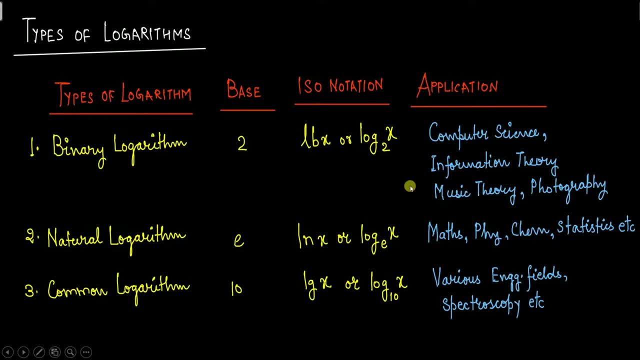 in which this logarithm is being applied. So what are the areas in which this logarithm is being applied? So I have written all these things such that you should have a fair idea that what is the purpose of studying logarithms. All right, So first type of binary logarithm. First type of logarithm: 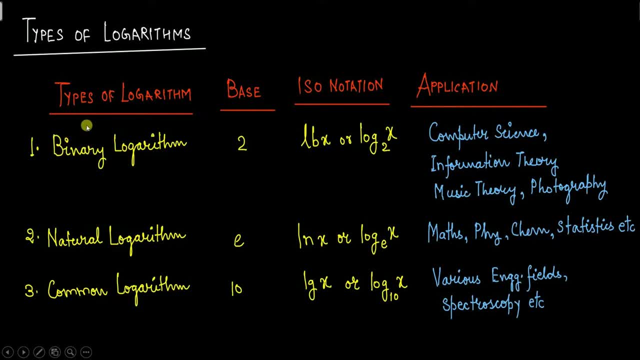 is binary logarithm. What is binary Bi means 2.. Okay, So binary logarithm, a logarithm in which the base is 2.. If your base is 2, so that is considered as binary logarithm. So what is the? 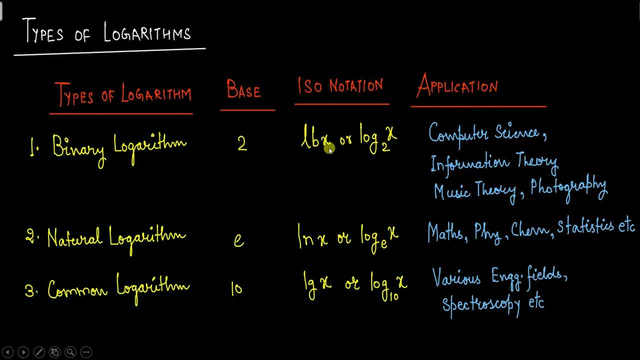 ISO notation, given It is LBX. Remember it is LBX. Or you can write this as log X to the base 2.. So log X to the base 2,, in short, is written as LBX. Till now we were just familiar with LNX or log X, But this is a new term for you, So please. 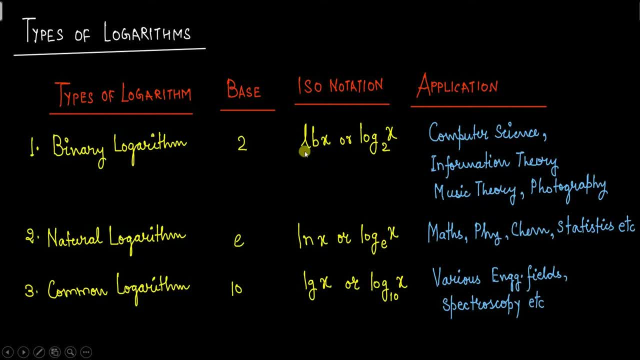 remember. this is very interesting. You can write here LBX. Okay, So LBX means log X to the base 2.. Where is it being applied? It is being applied in computer science, information theory, music theory, photography- Yes, photography, music theory- and so many wide applications it has got. 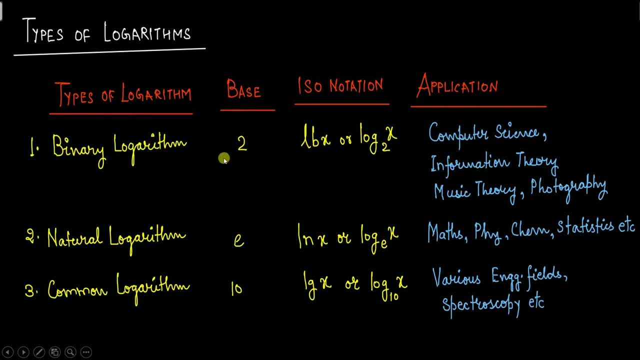 So basically these are things that are being applied in using the softwares, in the inside the softwares. Okay, So first type of logarithm is binary logarithm- Clear. Come to second type of logarithm. Second type of logarithm we have is natural logarithm. Second. 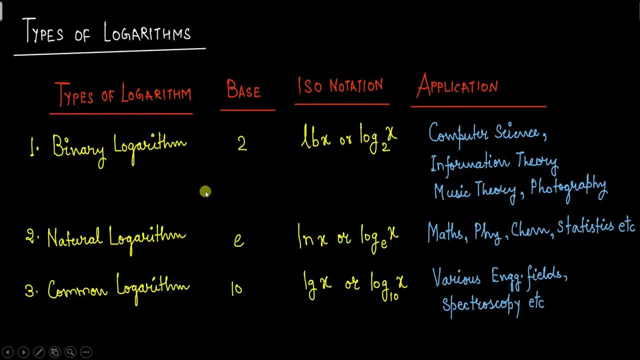 type of logarithm is natural logarithm. Here the base is E. What is this E? So we will see This is not a. this is an alphabetical letter, but it symbolizes a constant that we will see sometime later. So this is a constant. 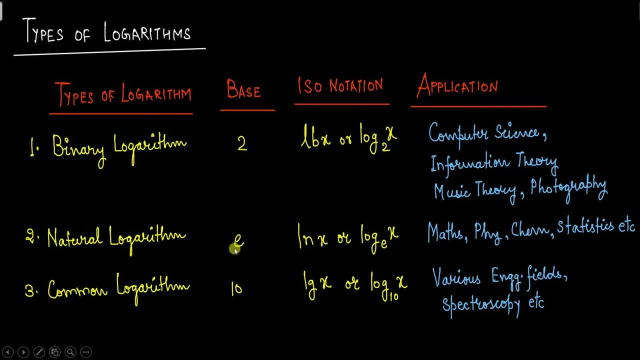 Okay. So this is not a variable, So this is a constant. So whenever the base is E, so that ISO notation is LNX, LNX means log X to the base E, Simple. So log X to the base E Whenever the base is considered as E. So in short, you can write like this: as LNX, Okay. 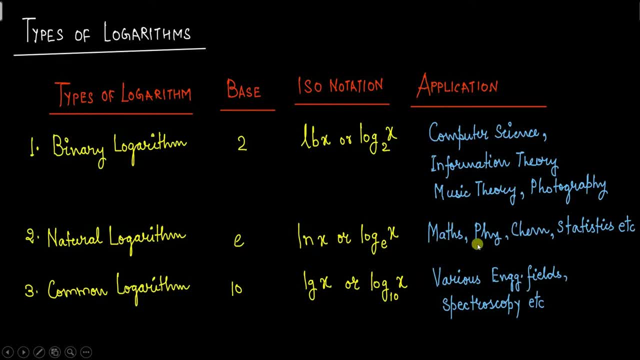 So what is the application for this Maths, physics, chemistry, statistics exercise? It also has got wide range of applications: Natural logarithm- You might be solving some numericals, or problems in your engine. You might be solving some problems in. 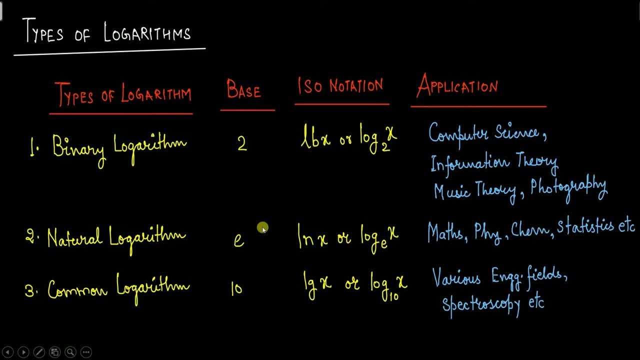 your engineering So you might be familiar with this term, right? So so many times this has come into picture by solving the problems. The third one, the most common one: common logarithm If the base is considered as 10.. Okay, So that is called as the common logarithm. So ISO notation. 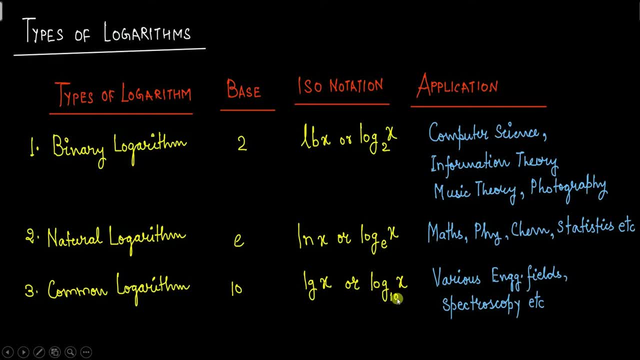 So you can write this as log X to the base 10, or this, in short, can be written as LGX. Remember So, initially, while we were pursuing our courses or your undergraduate courses, the most familiar terms that we were using was LNX and log X. Okay, So this LBX term is a new term. 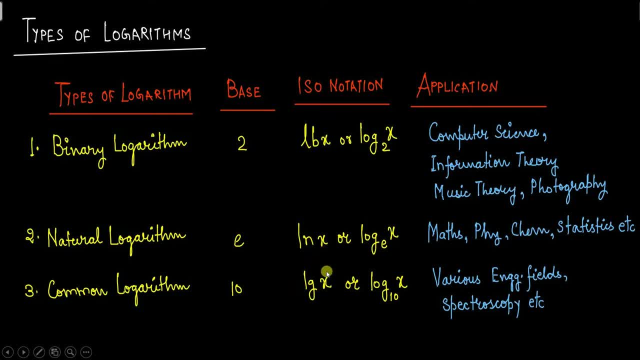 LGX is term. LGX is also a new term, So these are varieties of writing expressions with different ways of expressing the things. You can use whichever you want. So it has got a wide range of applications in various engineering fields: spectroscopy and so forth. Okay, Now one more. 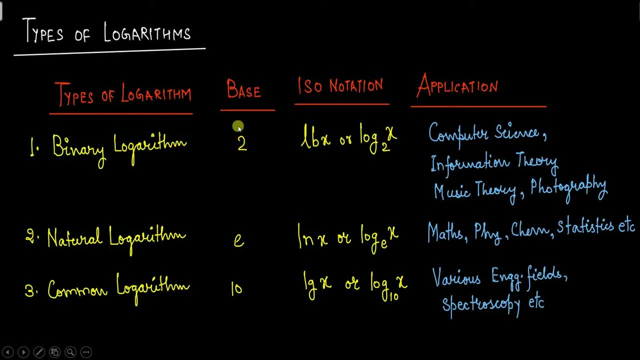 thing. So here I have shown only base 2, base E and base 10.. But this does not mean that you can use any base. It does not mean that a logarithm cannot have a base other than all these three. You can. 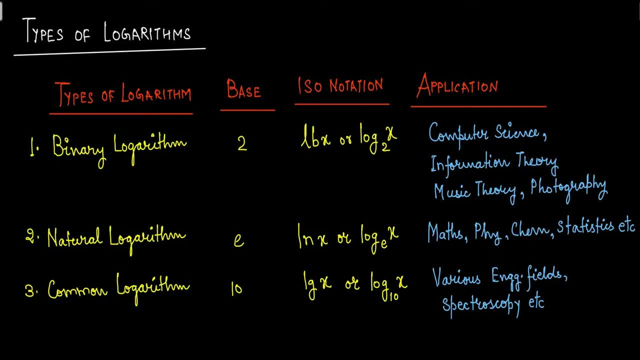 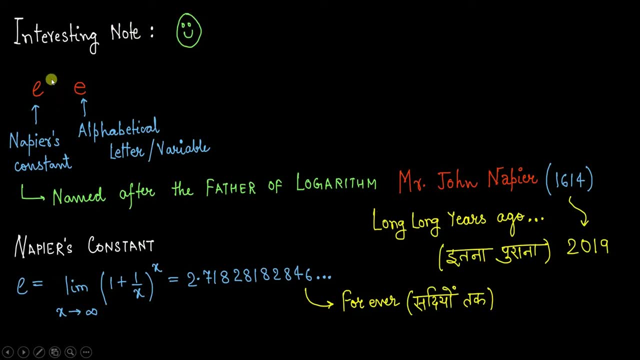 take any base, but the base should not be one. Remember that That's it. Let's have an interesting note. See two types of E. I'm seeing here two ways of writing E. So this is E. Take out your calculator, whichever scientific calculator you have, In that you might be having these two. 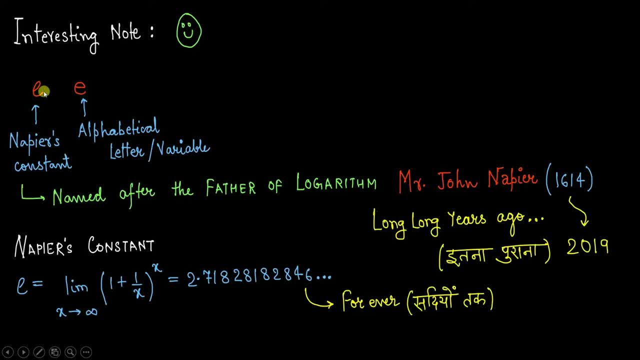 letters, One thing written in italics and one thing written like this. Okay, So this is simply a mathematical letter and it is a variable, And this whatever is written in italics. So this is called a Napier's constant. It is named after the father of logarithm, Mr John Napier. So Mr John, 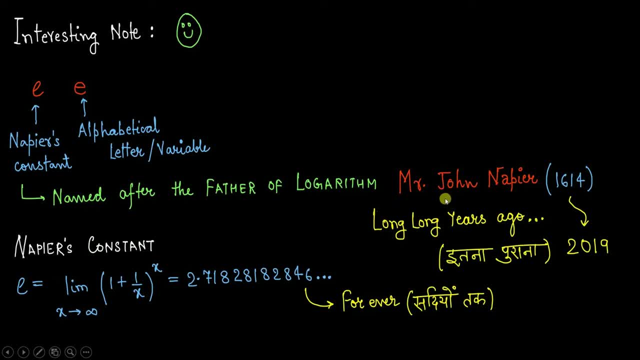 Napier was a mathematician, He was a professor. So just after his name, just in order to honor him, this constant is named after him, So which is called Napier's constant, Fine. So just see the year in which he discovered this. He just gave this term. He gave this term in 1614.. Long, long. 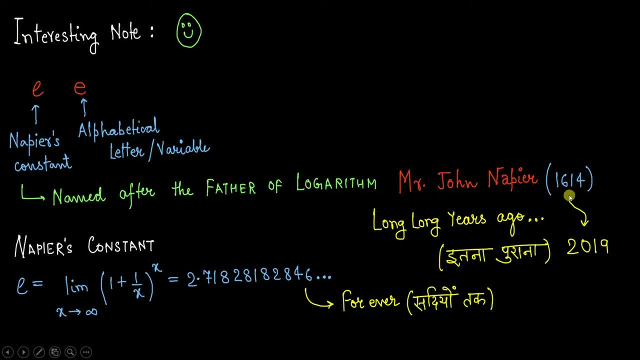 years ago, isn't it So long years ago? this concept has been coming and we have been using it currently. Okay, So what is this Napier's constant? So this is the definition for the Napier's constant. So this Napier's constant is defined as the limiting value of 1 plus 1 by x, whole raised to the power of x. 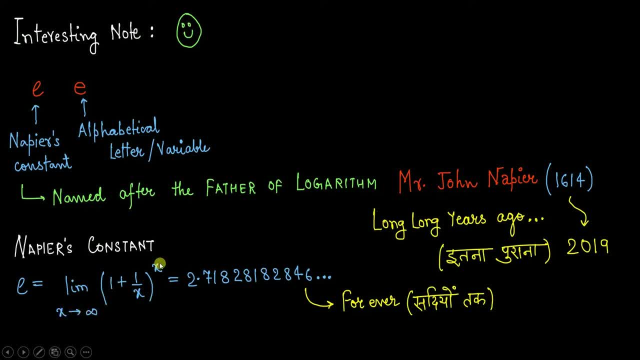 as x tends to infinity. Okay, So this is the definition for this Napier's constant. And what is the value for this? When you will press in calculator so you'll get 2.71828.. 8182846, and so on, So it will go on forever, forever. So it is a recurring, Okay, Non-repeating. 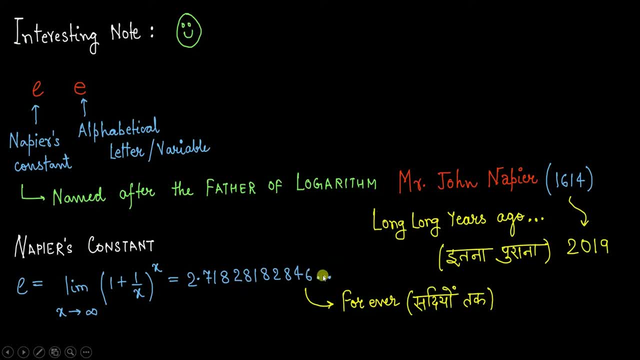 but recurring, It is continuous. It can never stop. It is going continuously. Okay So, but for our approximation we take it as 0.271 or 2, sorry, 2.718 for our calculations. Got the idea. 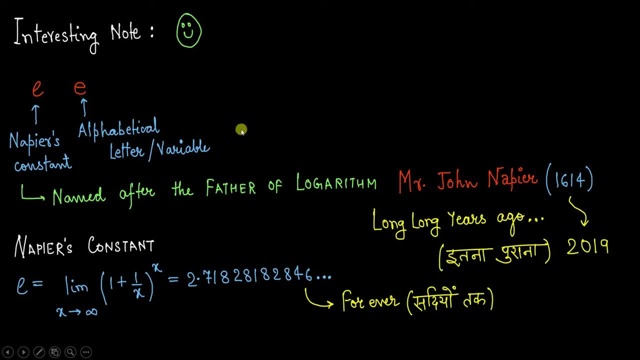 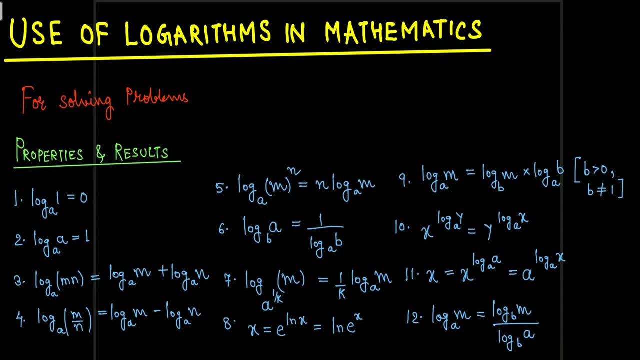 What is this? Napier's constant? Okay, Now, finally, the question comes, sir: how to use this logarithms in mathematics for solving problems. Definitely, we'll be using this logarithms for solving the problems. So what? there are some properties and results that you should learn. 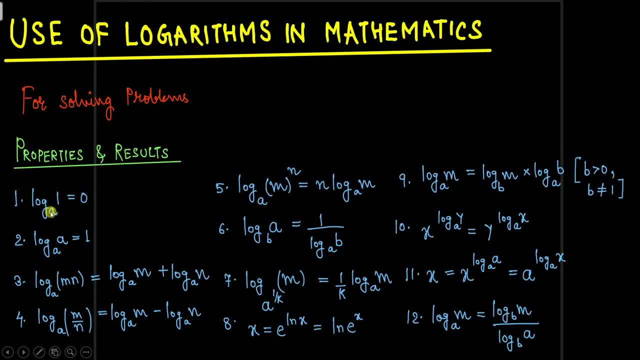 these properties by heart. Okay, So let's see what is the first property. First property is log 1 to the base. a is 0.. Log 1.. Okay, So, log 1,. whichever base you take, that will be 0.. 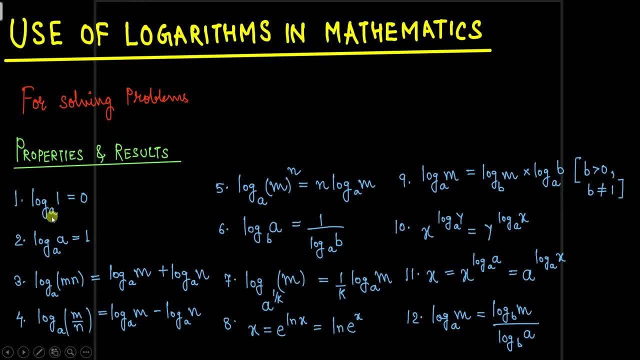 Okay, No problem. So log 1 to the base a is always 0. Then log a to the base a is 1.. Log a to the base a is 1.. Why is it log a to the base a is 1? Because log a to the base a. 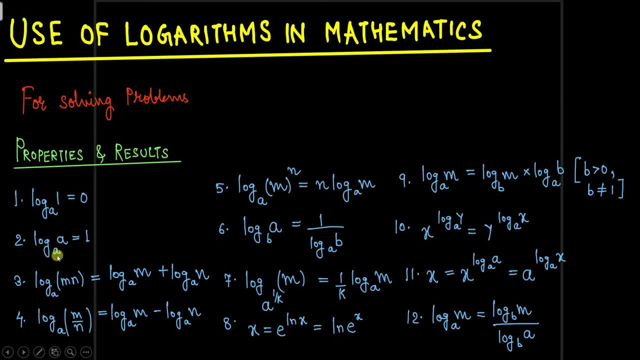 you can write this as log a upon log a. So log a, log a, gets cancelled, and this could be written as: 1. The third property that we are seeing here. this third property log mn to the base a. So whenever you find any product of two variables, so log gets separated and gets added. 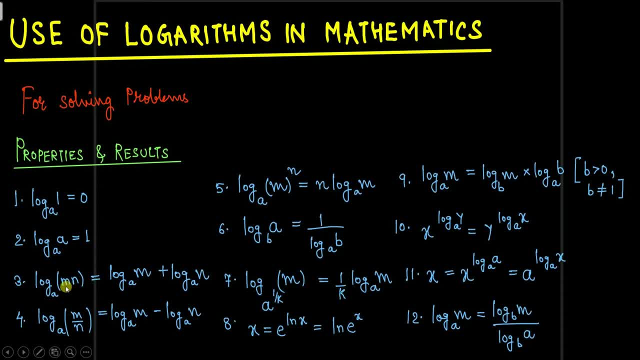 So log m to the base a plus log n to the base a. Okay, So whenever there is any product of two variables, the log gets added. Similarly, whenever there is a division of two variables, the log gets separated and base remains same. 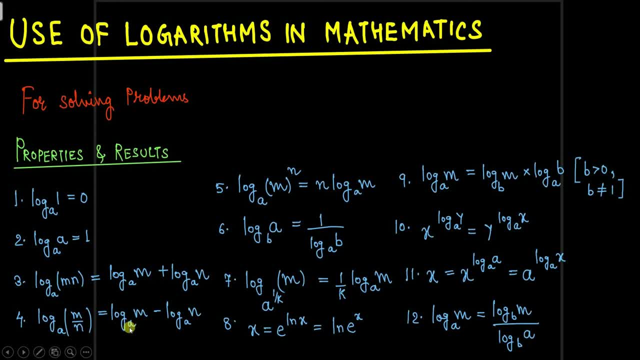 So this gets distributed here. So log m to the base a minus. log n to the base a Clear All these four properties, moving to number 5.. So whenever you see that we have log m to the power n and base a, So as we can see that whatever is written in power that will come on the left hand, 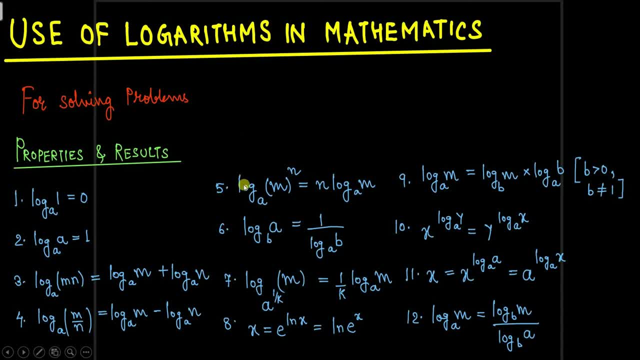 side. This will come on the left Left hand side of it, So this could be written as n. log m to the base a, So fifth property is also clear. Coming to sixth property, So log a to the base b. So this could be written as 1 upon log b. 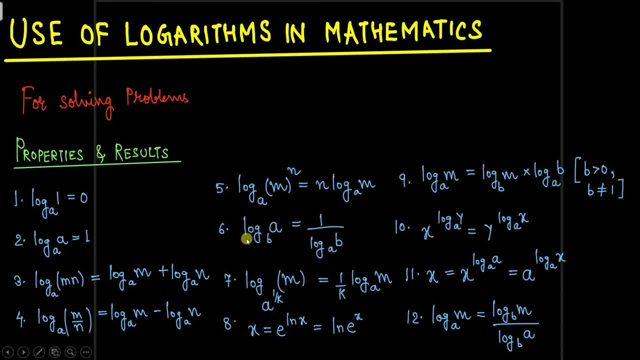 to the base a. This could be written as 1 upon log b to the base a. So it becomes reciprocal Whenever you are interchanging the base and the base with this variable. so it gets that reciprocal, It gets converted into a reciprocal. 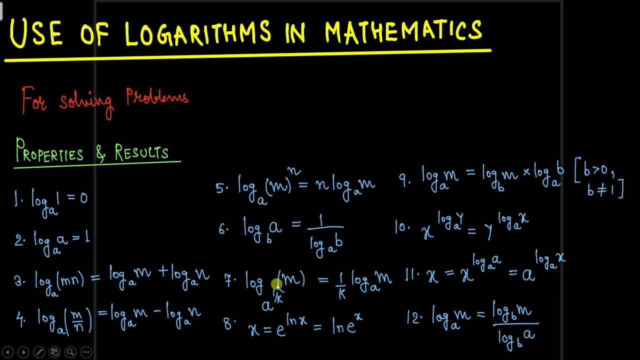 So log m to the base a to the power: 1 by k. Now this could be written as 1 by k. log m to the base a. This you can do it from all the properties. Now x equals to e to the power of ln. x. Now e to. 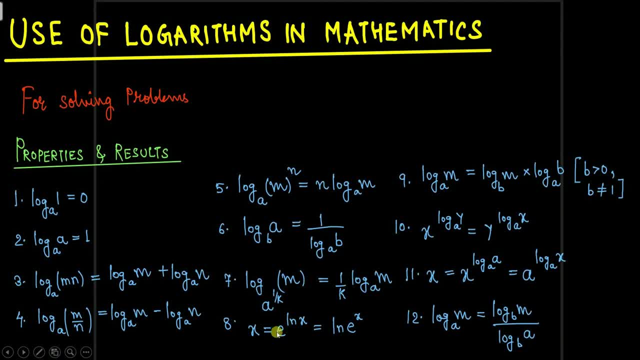 the power of ln x. So if you take the log on both the sides I am taking natural logarithm on both the sides. So here if I write ln x, this will be ln e to the power of ln x And this ln x will. 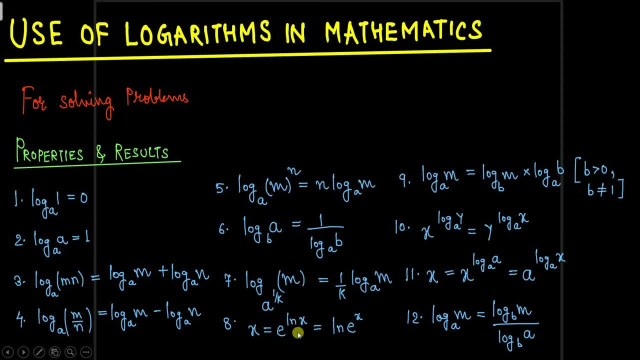 come on the left hand side and ln e is 1.. So this will get converted Ln e to the power of x. Fine, Coming to ninth property, we have log m to the base a equals to log m to the base b into log b to the base a. So we can write this format simply. 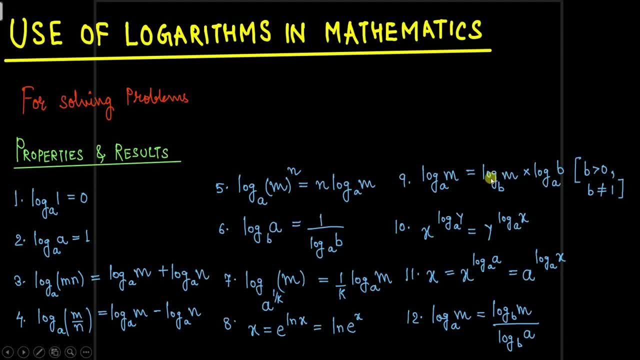 That. it simply means that you can write this as log m to the base a multiplied with log b to the base a, So log b log b gets cancelled and it again finally becomes log m to the base a, provided your b value is greater than 0 and b is not equal to 1.. Okay, Coming to number 10, we have a measure of 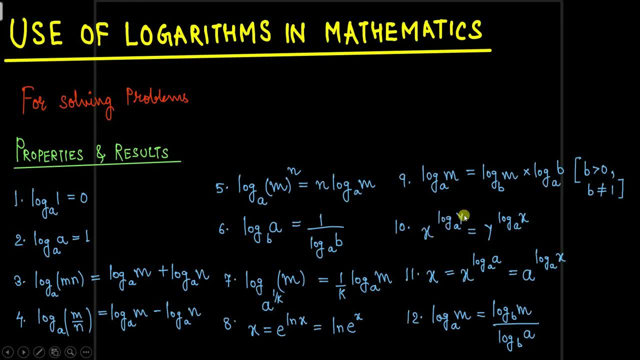 log m to the base a, which is minus 1.. So this is not equal to 2 mod n e to the base a. Now, if you have x equals to x to the power of log y to the base a equals to y to the power of log x to the. 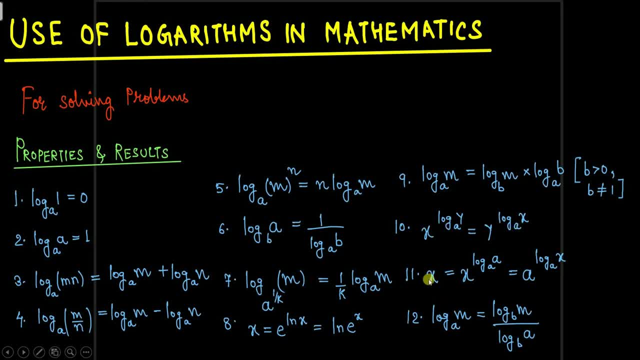 base a. simply you can interchange like this number. 11th property: we have x equals to x to the power of log a to the base a equals to a to the power of log x to the base a. simply you can derive all these expressions from the previous properties. but i will recommend you, i will suggest you to 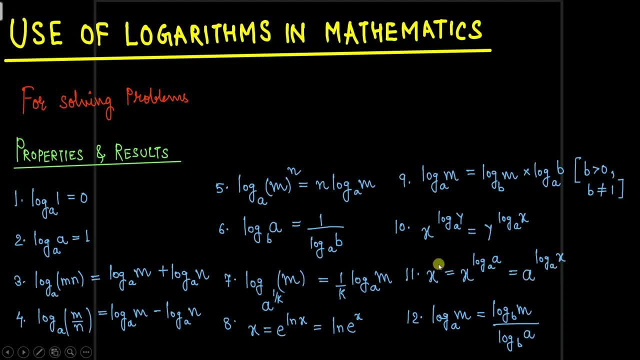 kind of learn all these properties by heart, because in the examination you don't have that much of time to derive the things right. so remember all these properties by heart now. last property that we have is log m to the base a equals to log m to the base b divided by log a to the 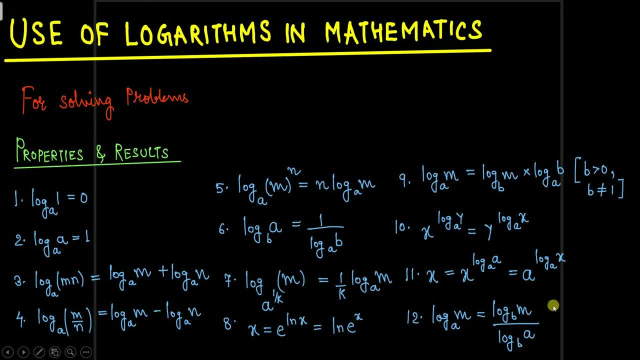 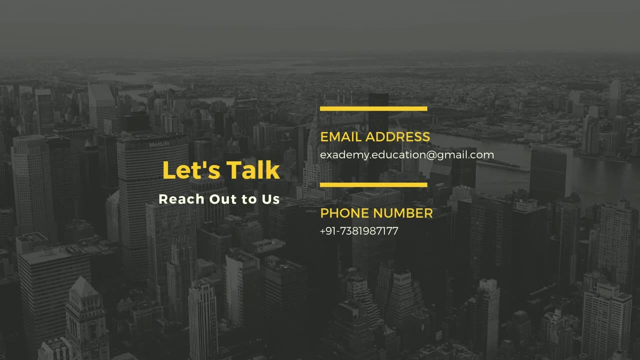 base b. okay, so with this we have completed our second topic, that is, logarithms. so in the third topic we'll be seeing something else. till then, take care, bye you.